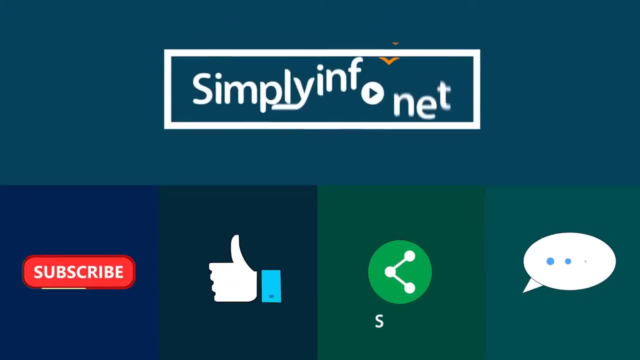 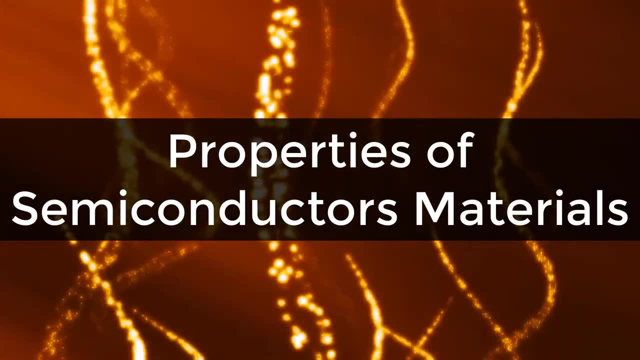 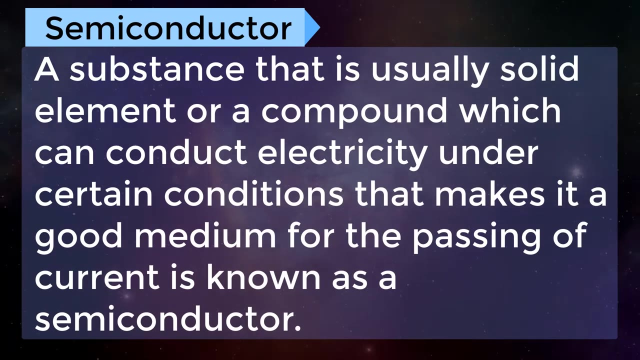 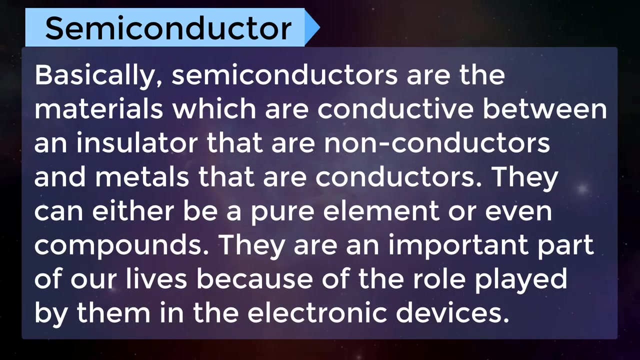 Properties of Semiconductor Materials. Semiconductor Definition: A substance that is usually solid element or a compound which can conduct electricity under certain conditions that makes it a good medium for the passing of current, is known as a semiconductor. Basically, semiconductors are the materials which are conductive between an insulator and are non-conductors. 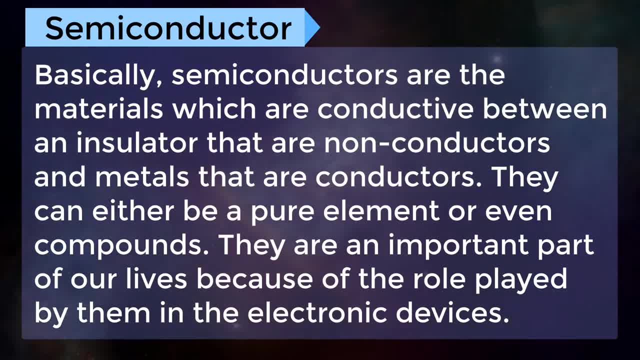 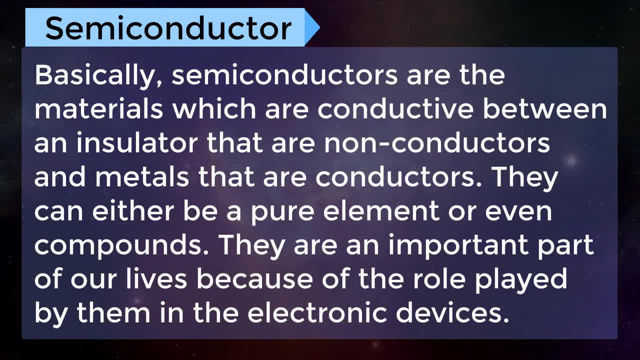 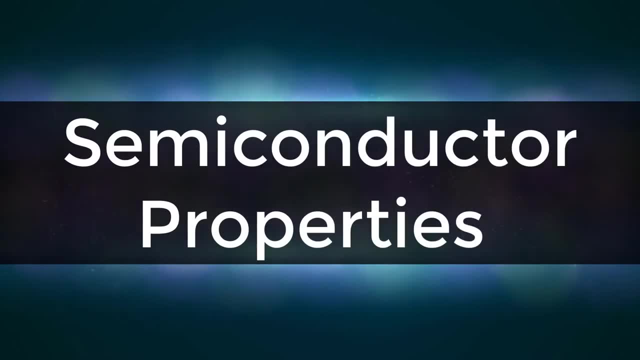 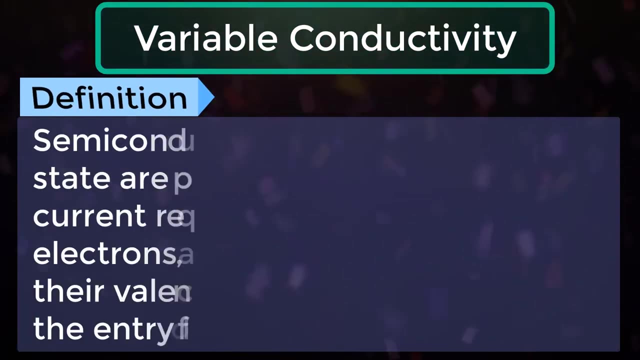 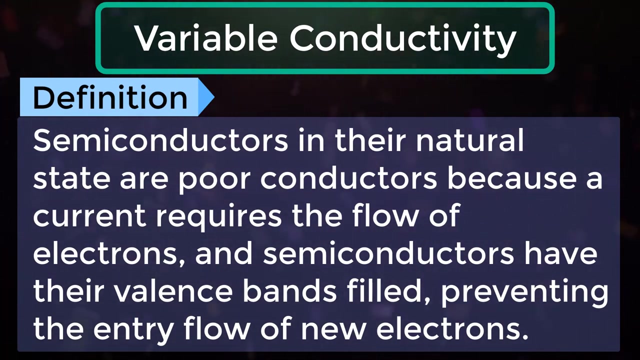 and metals that are conductors. They can either be pure element or even compounds. They are an important part of our lives because of the role played by them in the electronic devices. Semiconductor Properties. Semiconductor Properties- Semiconductors in their natural state are poor conductors because a current requires the flow of electrons and semiconductors have their valence bands filled, preventing the entry flow of new electrons. 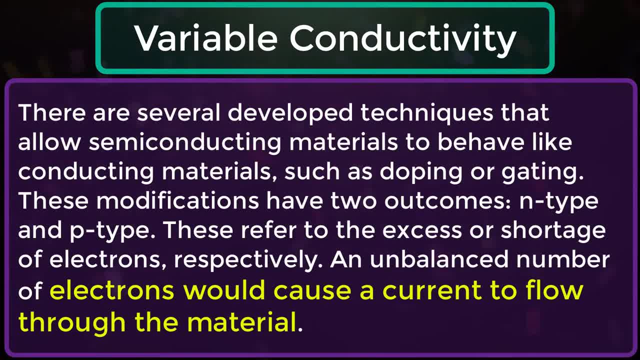 There are several developed techniques that allow semiconducting materials to behave like conducting materials, such as doping or gating. These modifications have 2.. There are two outcomes: n-type and p-type. These refer to the excess or shortage of electrons respectively. 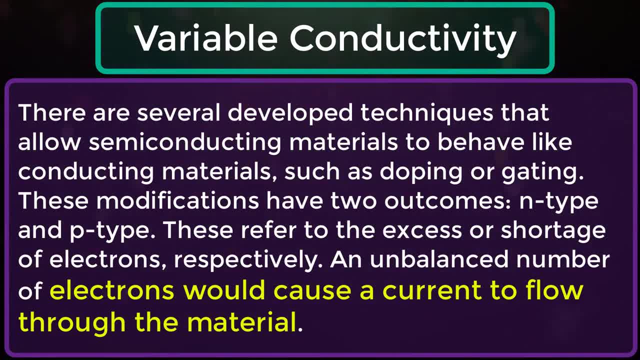 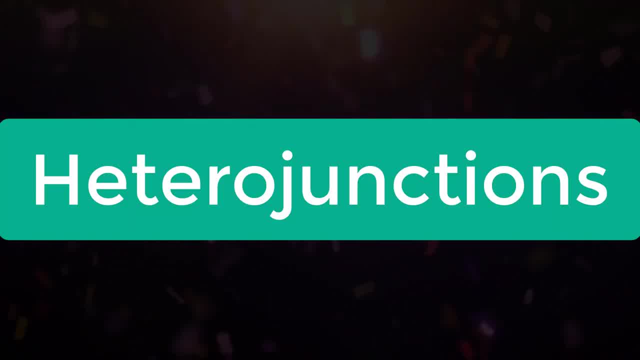 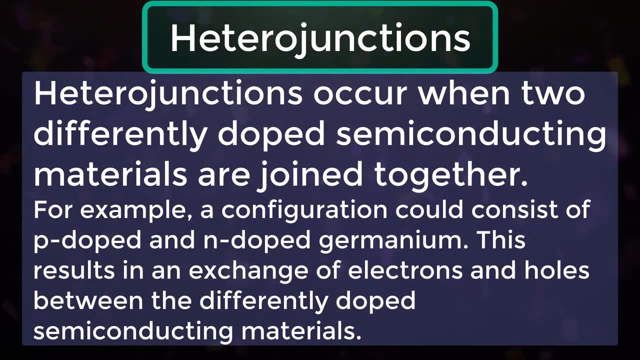 An unbalanced number of electrons would cause a current to flow through the material. Heteronucleotides. Heteronucleotides occur when two differently doped semiconducting materials are joined together. For example, a configuration could consist of p-doped and n-doped germanium. 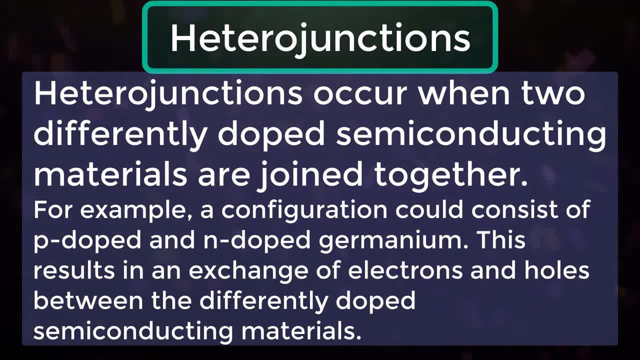 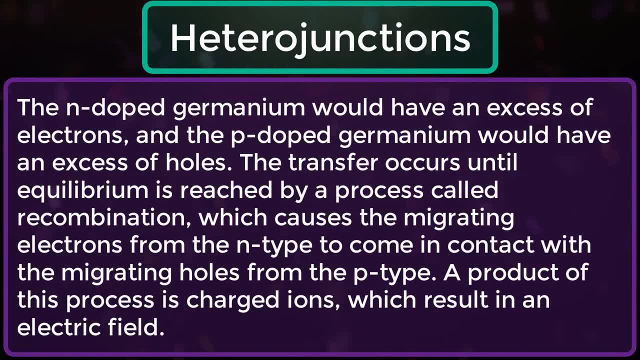 For example, a configuration could consist of p-doped and n-doped germanium. This results in an exchange of electrons and holes between the differently doped semiconducting materials. The n-doped germanium would have an excess of electrons and the p-doped germanium would have an excess of holes. 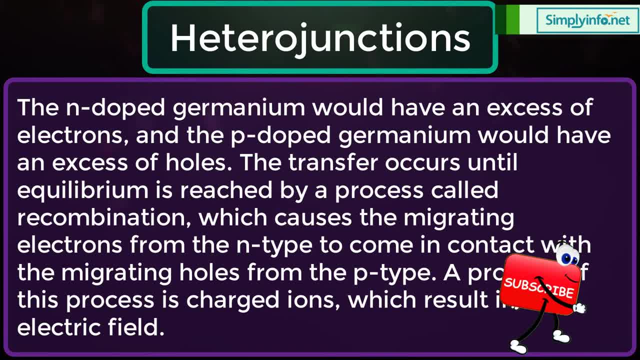 The transfer occurs until equilibrium is reached by the process called recombination, which causes the migrating electrons from the n-type to come in contact with the migrating holes. which causes the migrating electrons from the n-type to come in contact with the migrating holes. which causes the migrating electrons from the n-type to come in contact with the migrating holes.